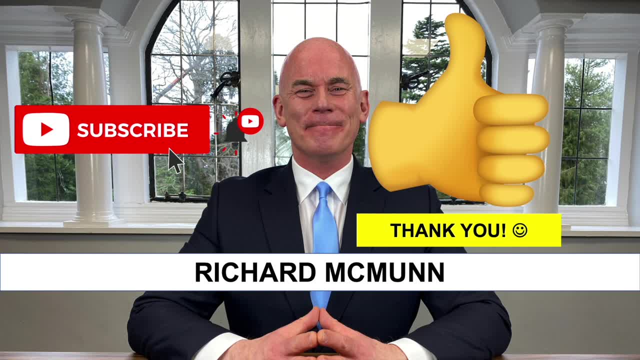 these tutorials useful and it motivates me to create more content for you, So please subscribe to my YouTube channel And I will see you in the next video. Bye, bye. Okay, So the first construction manager interview question I recommend you prepare. 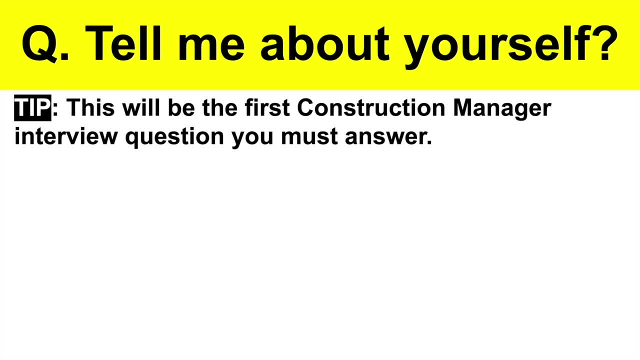 for is tell me about yourself. So this is going to be the first question, the first interview question that you must answer. So I recommend talking about the skills, qualities and experience you have. that will add value to their organization if they hire you. I. 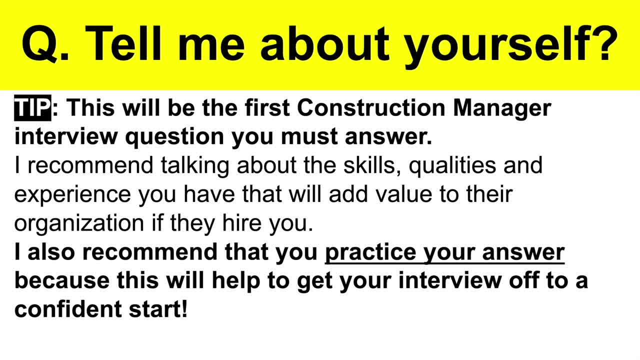 also recommend that you practice your answer to this question, because this will help to get your interview off to a confident start. Remember, this is the first question you will have to answer. You will most likely be the most nervous right at the very start. 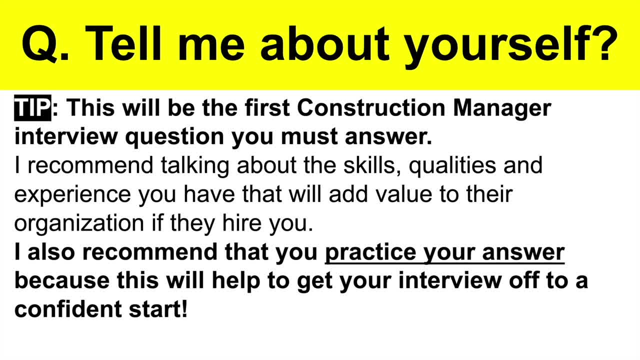 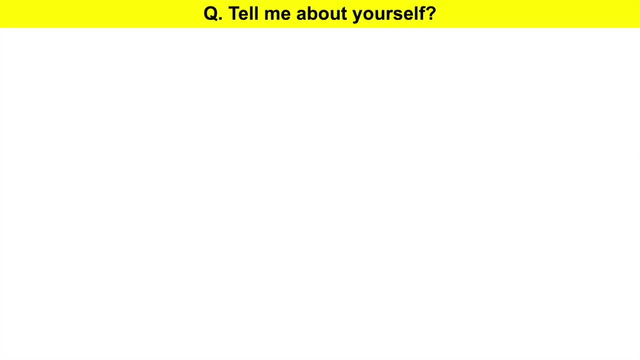 But if you give a confident response, it really sets you up for the rest of your interview. So to help you, let me give you a brilliant example: answer: Tell me about yourself. Here we go. Thank you for giving me the opportunity to be interviewed for this construction manager. 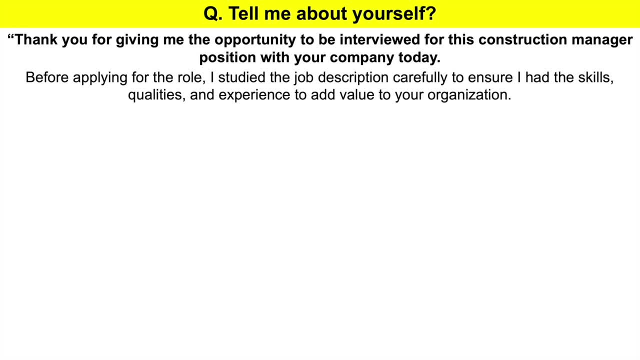 position with your company today. Okay, Before applying for the role, I studied the job description carefully to ensure I had the skills, qualities and experience to add value to your organization. I would describe myself as a technically astute, confident, knowledgeable and industrious construction. 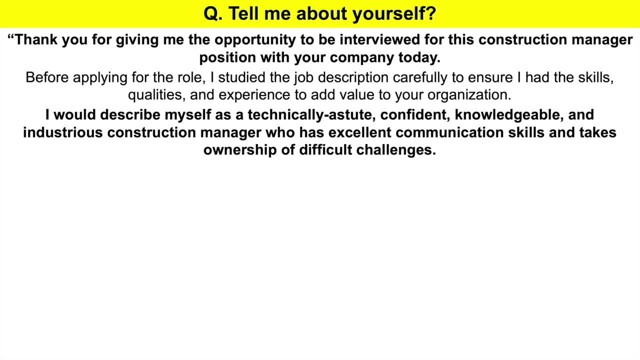 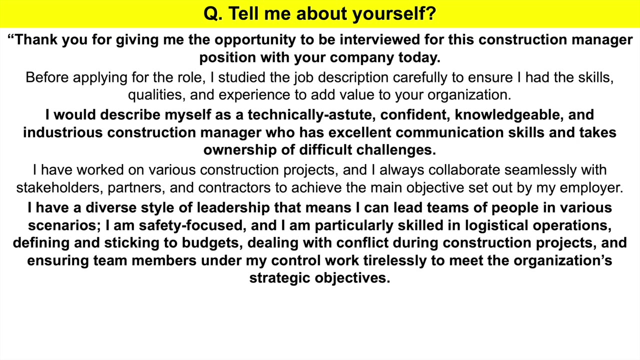 manager who has excellent communication skills and takes ownership of difficult challenges. I have worked on various construction projects and I always collaborate seamlessly with stakeholders, partners and contractors to achieve the main objectives set out by my employer. I have a diverse style of leadership that means I can lead teams of people in various 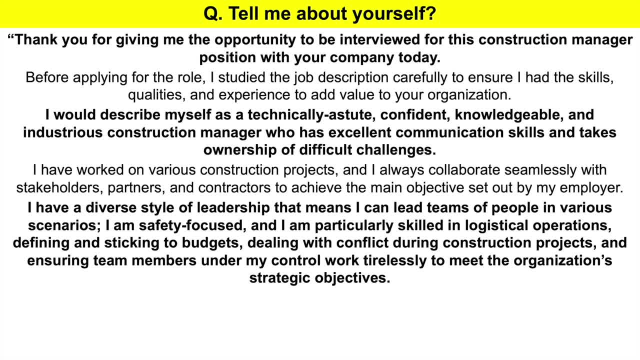 scenarios. I am safety-focused and I am particularly skilled in logistical operations, defining and sticking to budgets, dealing with conflict during construction projects and ensuring team members under my control. I am also an expert in the construction industry and I have worked in the construction industry for many years. I have worked in the construction. 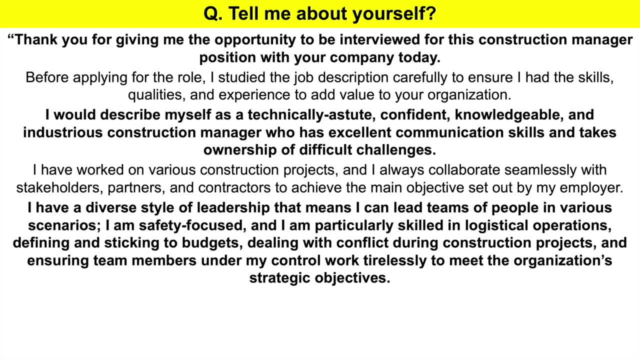 industry for many years. I have worked tirelessly to meet the organization's strategic objectives. If you hire me as your construction manager, it will be my focus to deliver exceptional value for money in the role and ensure consistently strong results during projects are achieved. That is a brilliant answer to that first construction manager interview question. Tell me about. 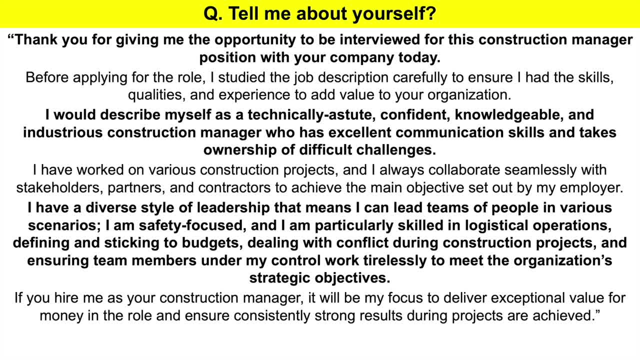 yourself. Now. you can either pause the video, if you want to, and take a note of the question And answer as we work through them together, Or, if you want to wait, I will soon tell you where you can instantly download my full set of 22 construction manager interview questions. 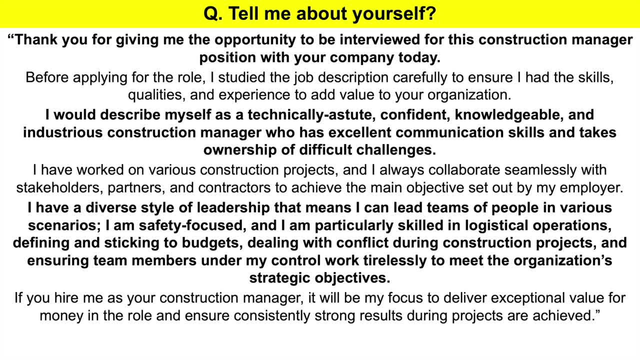 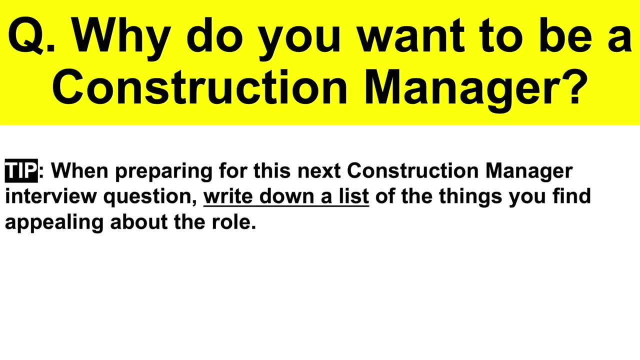 and top scoring example answers, including the ones we are working through together today. But here's the next question for you: Why do you want to be a construction manager? Now, when preparing for this next interview question, my advice is to write down a list. 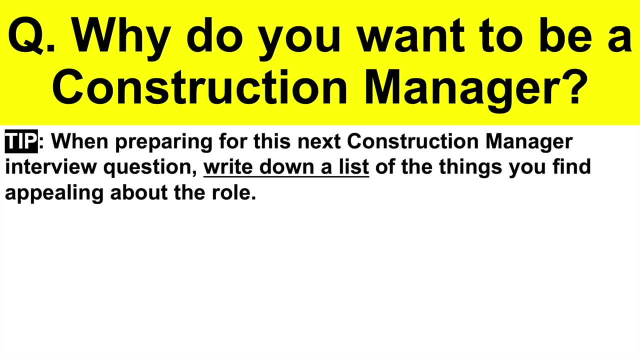 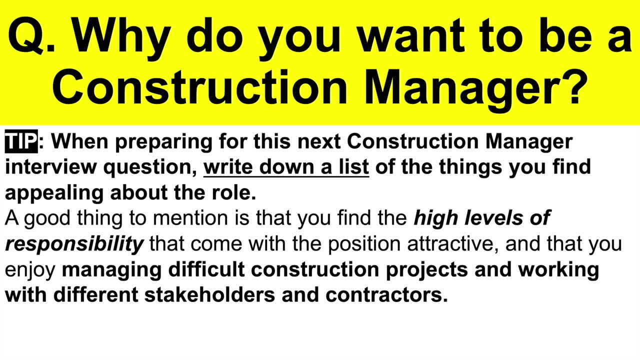 of the things you find appealing about the role of a construction manager. Now, a good thing to mention is that you find the high levels of responsibility that come with the position attractive and that you enjoy managing difficult construction projects and working with different stakeholders and contractors. Here's another great example. answer to help. 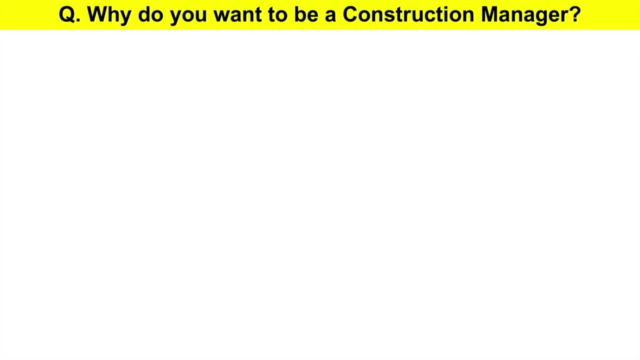 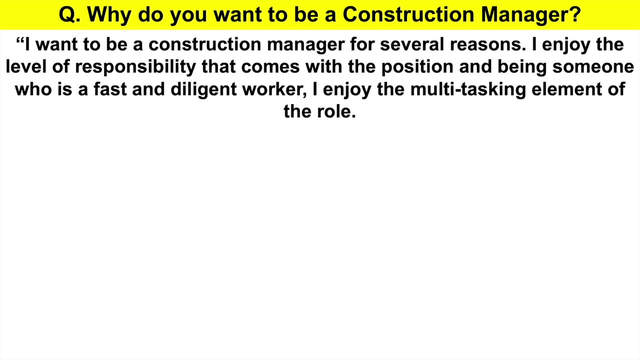 you. Why do you want to be a construction manager? Here we go. I want to be a construction manager for several reasons. I enjoy the level of responsibility that comes with the position and being someone who is a fast and diligent worker. I enjoy the multitasking. 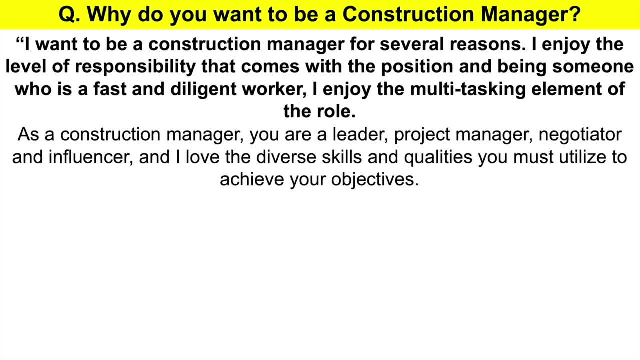 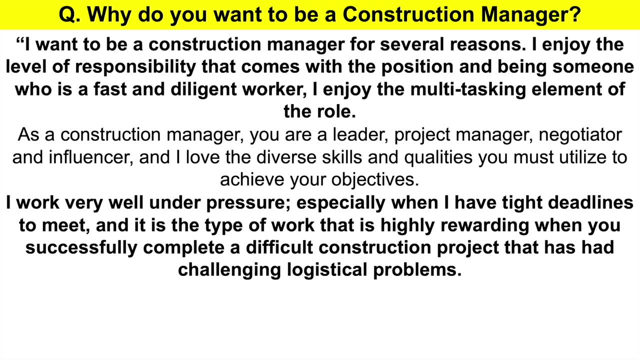 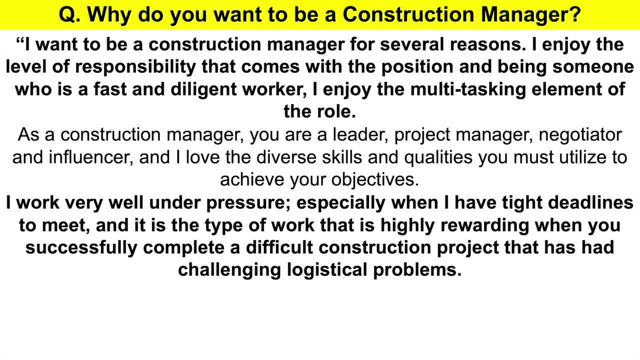 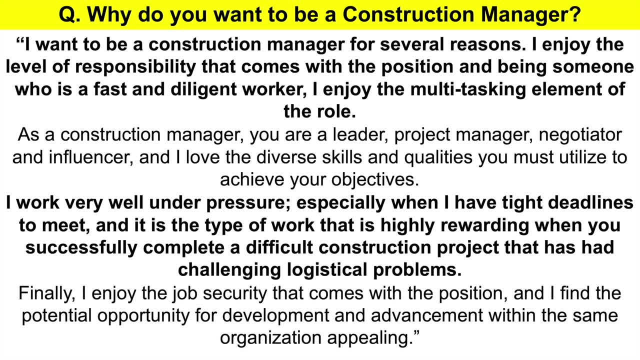 best for you. You deserve the award that was back then And I want to overcome any goal, especially if you think that it's environments to hire killer and don't take your credit cards too far. It's best if you are being your goals. You are worthy of what you want to be, What you're- half Jarois Jason's. 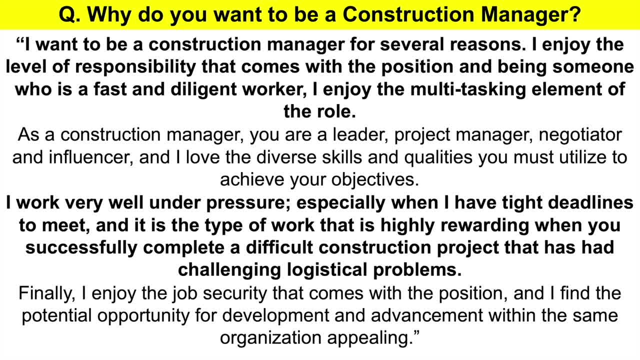 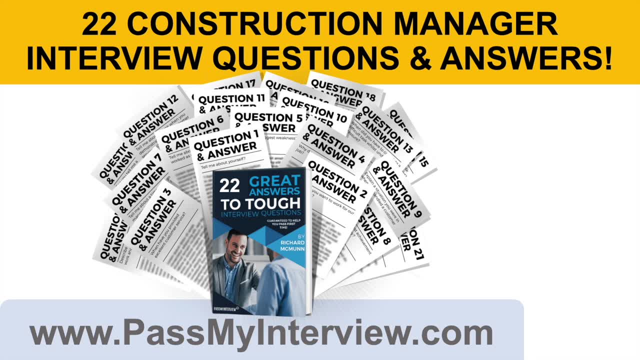 platform isAll about. is the or лишables, thinking of creating your goals. reject, nee, taking no chances. The skill, because I still have more questions and answers to work through with you. But when you're ready, click that link in the top right hand corner of the video and you can head through to my website. 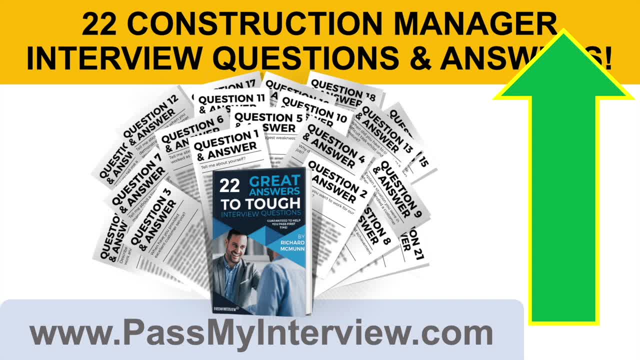 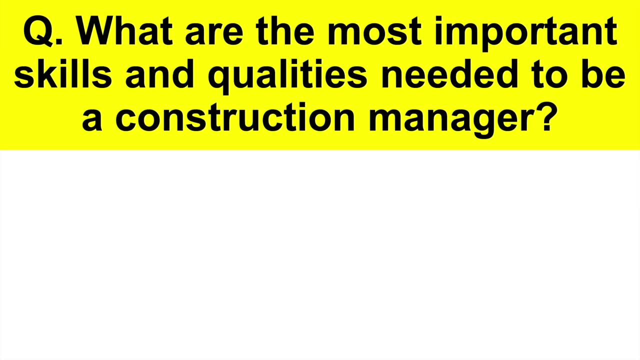 PassMyInterviewcom and you can instantly download my full set of 22 Construction Manager interview questions and top scoring answers, including the ones we are working through together today. But here's the next question for you: What are the most important skills and qualities needed to be a Construction Manager? Now, this interview question is assessing your 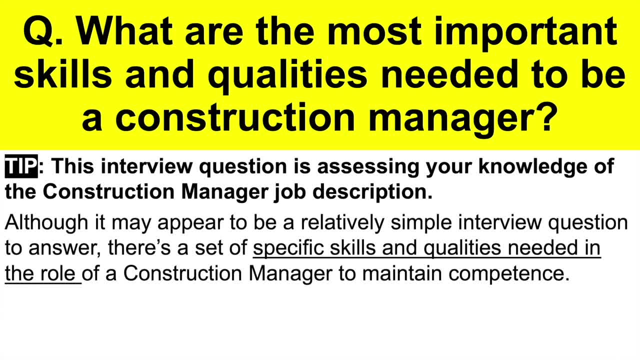 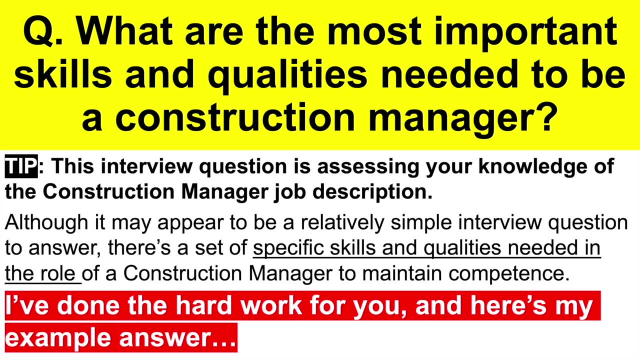 knowledge of the job description? Now, although it may appear to be a relatively simple interview question to answer, there's a set of specific skills and qualities needed in the role to maintain competence. Now I've done all the hard work for you and here's my example answer. 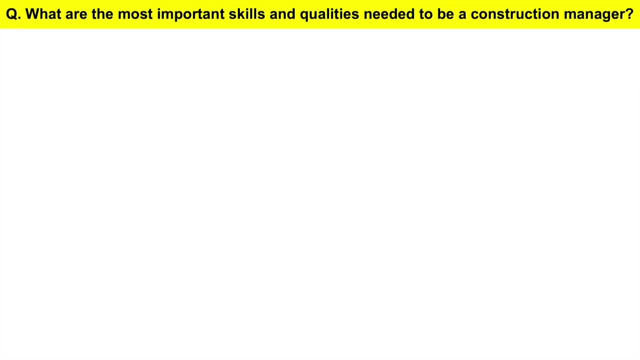 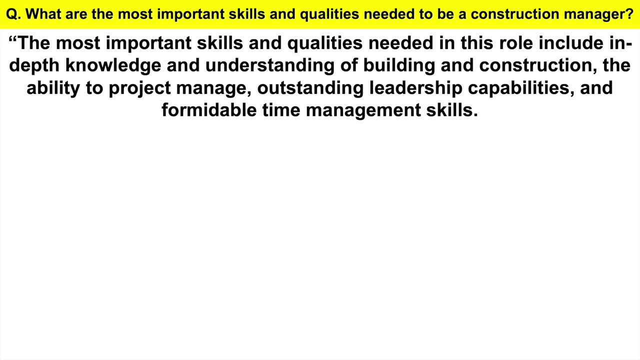 What are the most important skills and qualities needed to be a Construction Manager? Here we go. The most important skills and qualities needed in this role include in-depth knowledge and understanding of building and construction, the ability to project manage, outstanding leadership capabilities and formidable time management skills. 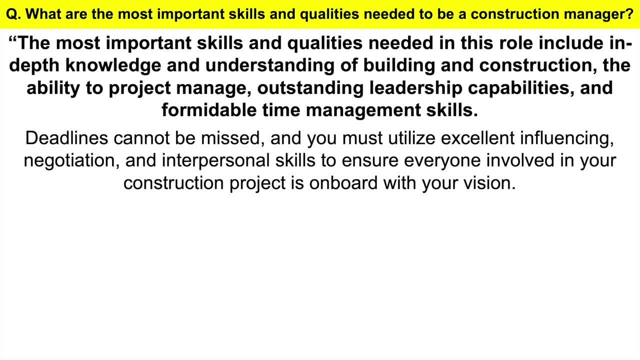 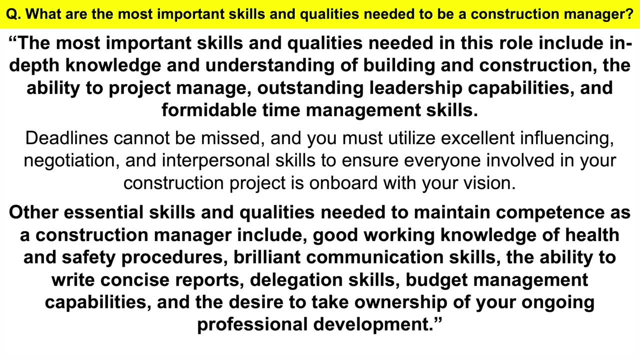 because deadlines cannot be missed and you must utilize excellent influencing, negotiation and interpersonal skills to ensure everyone involved in your construction project is on board with your vision Now. other essential skills and qualities needed to maintain competence as a Construction Manager include good working knowledge of health and 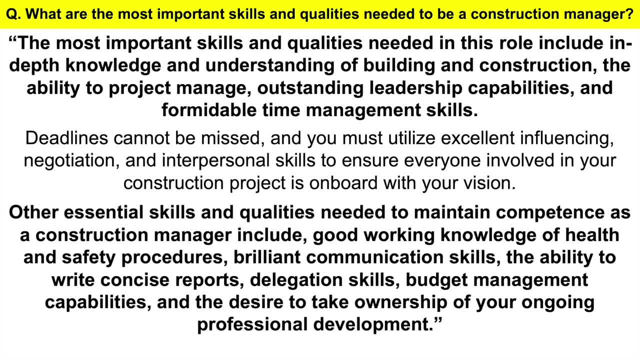 safety procedures, brilliant communication skills, the ability to write concise reports, delegation skills, budgeting management capabilities and the desire to take ownership of your ongoing professional development. That is another. Now the next question is a brilliant, positive and top-scoring answer that's going to help. 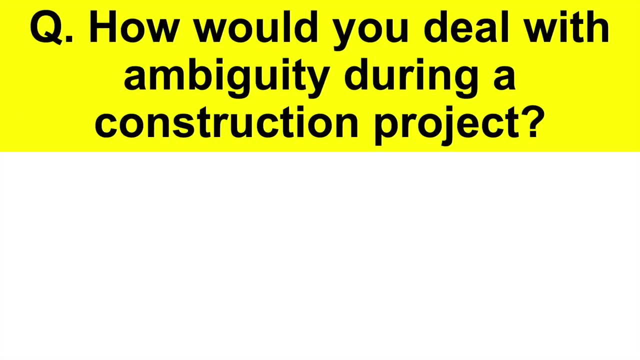 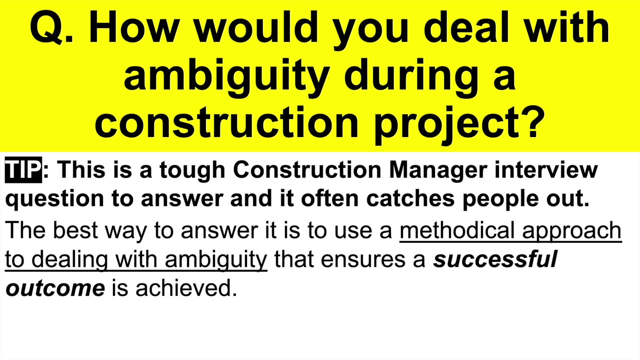 you be the standout candidate. Here is the next question: How would you deal with ambiguity during a construction project? These questions are starting to get difficult now. This is a tough interview question to answer and it often catches people out: Now the best. 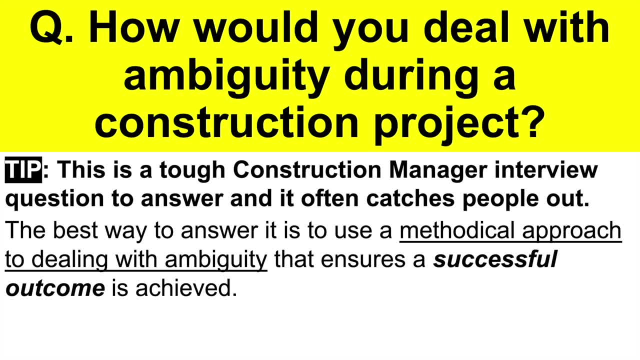 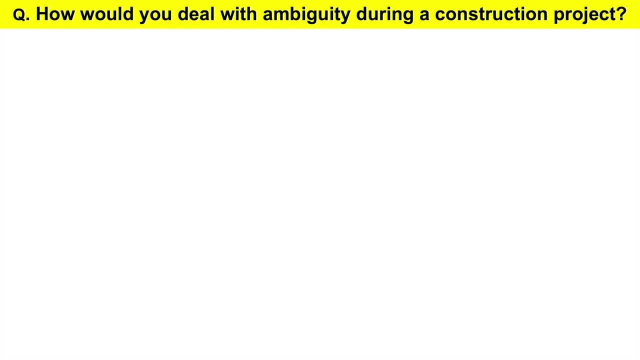 way to answer it is to use a methodical approach to dealing with ambiguity that ensures a successful outcome is always achieved. Here's another great example answer to assist you. How would you deal with ambiguity during a construction project? Here's my example answer. 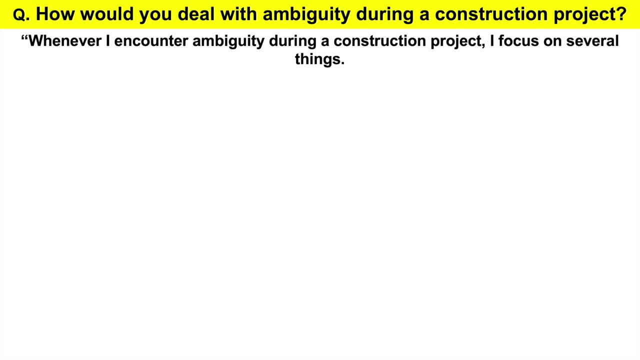 Whenever I encounter ambiguity during a project, I focus on several things. First, I determine the exact cause of the ambiguity. Is it the absence of key information, indecision, misinterpretation of the project's requirements or a conflict between team members? 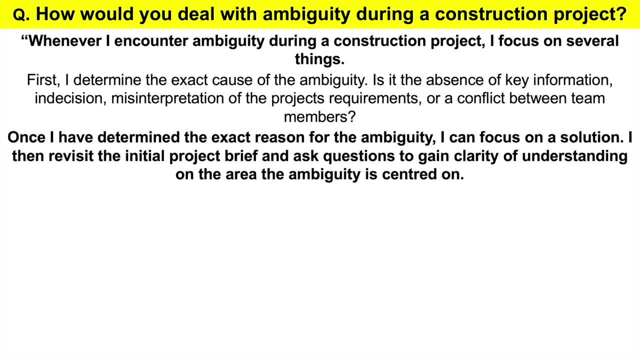 Now, once I have determined the exact reason for the ambiguity, I can then focus on a solution. I then revisit the initial project brief and ask questions to gain clarity of understanding on the area the ambiguity is centered on. For example, in a previous role I took over 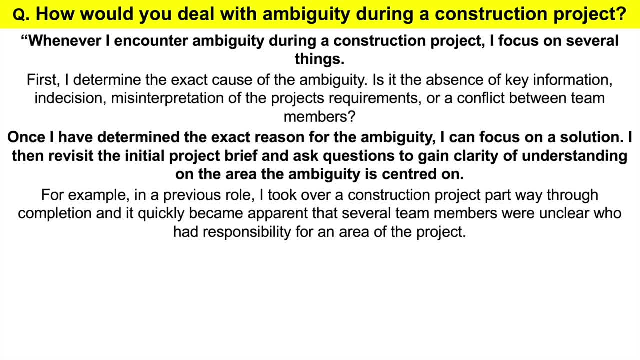 a construction project partway through completion and it quickly became apparent that several team members were unclear who had responsibility for ambiguity. I then asked them to provide an area of the project. The previous manager had assumed the team members would sort this out themselves, but that never happened. The conflict was having a detrimental effect on 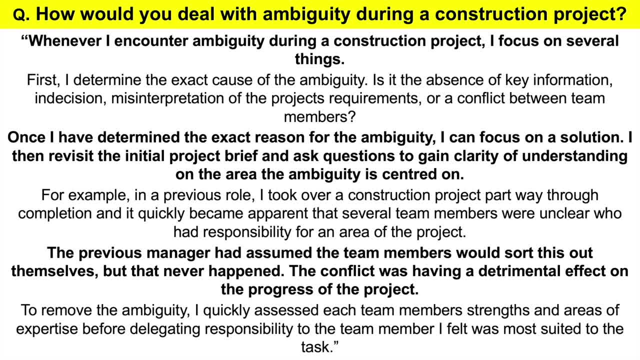 the progress of the project. To remove the ambiguity, I quickly assessed each team member's strengths and areas of expertise before delegating responsibility to the team member I felt was most suited to the task. That's a confident answer that definitely puts you across as a competent construction manager, because you can easily deal with ambiguity. 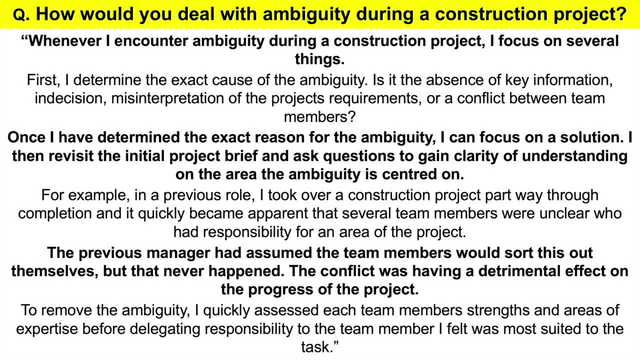 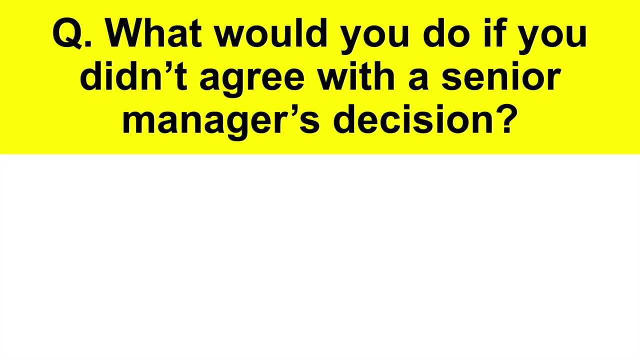 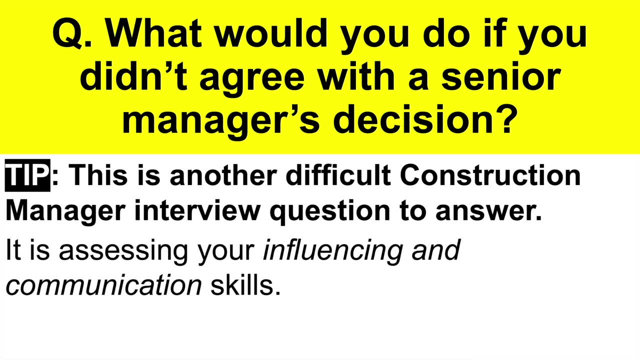 by following a methodical approach that guarantees a successful outcome. Here's the next question: What would you do if you didn't agree with a senior manager's decision? Now, this is another difficult construction manager interview question to answer. It is assessing your influencing. 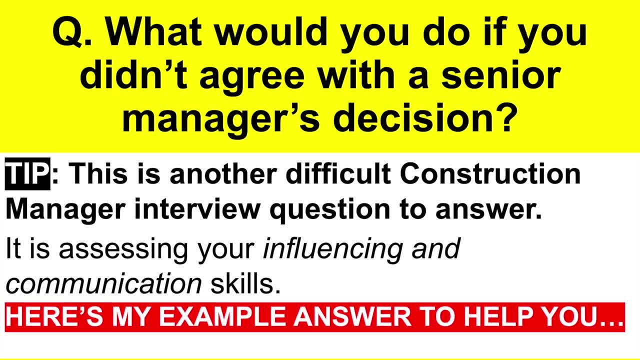 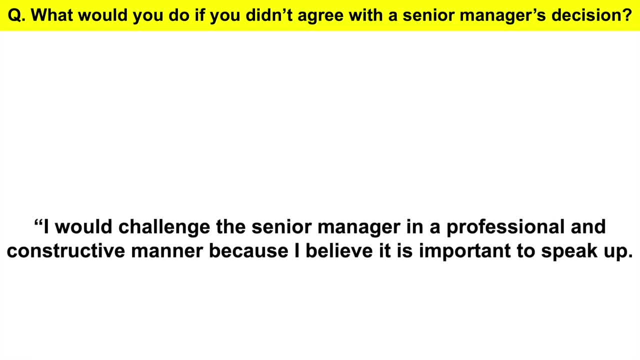 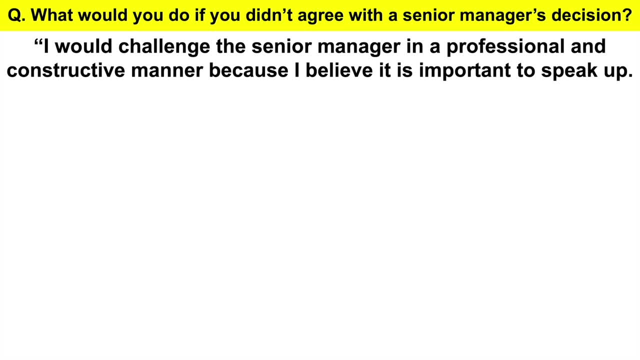 and communication skills. Here's my example answer to assist you. What would you do if you didn't agree with a senior manager's decision? Here we go. I would challenge the senior manager in a professional and constructive manner, because I believe it is important to speak up. If you don't speak up and give your 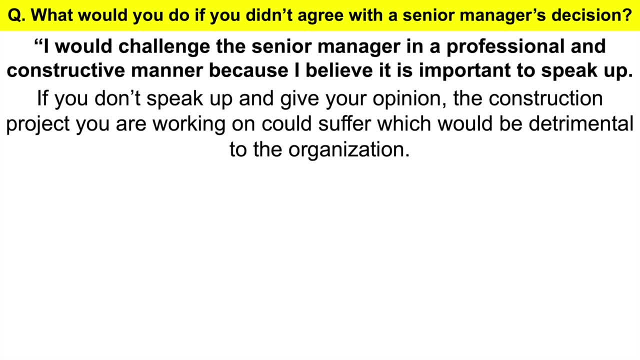 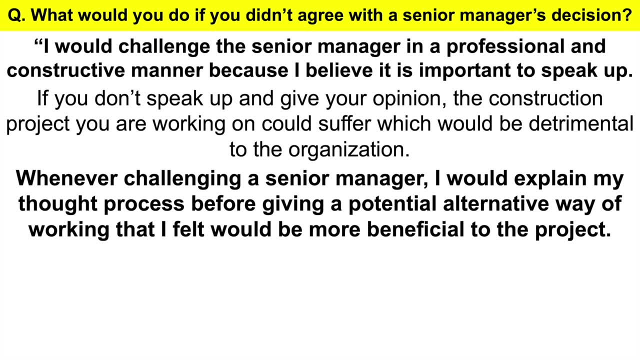 opinion, the construction project you are working on could suffer, which would then be detrimental to the organization. Now, whenever challenging a senior manager, I would explain the process before giving a potential alternative way of working that I felt would be more beneficial to the project. The senior manager would then have the additional information needed to. 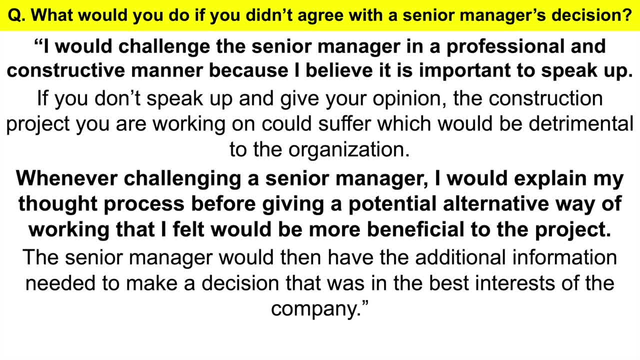 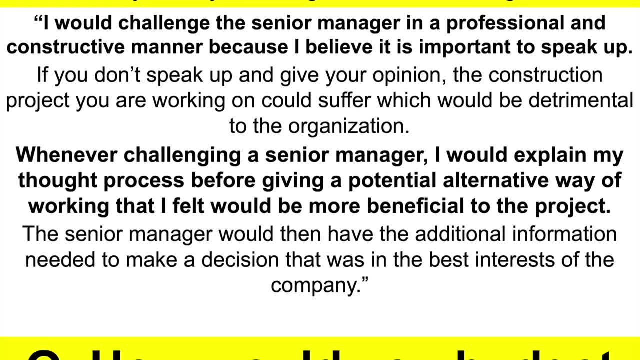 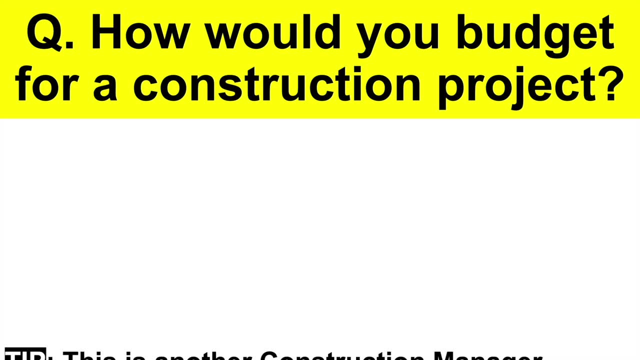 make a decision that was in the best interests of the company. That is a simple but concise answer that again shows you to be a competent construction manager. It's a great response. Now this is another really difficult one: How would you budget for a construction project? 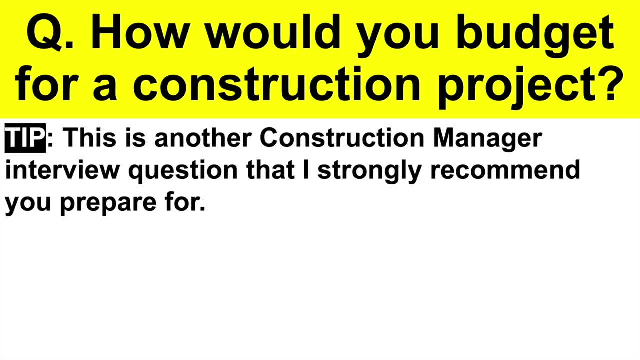 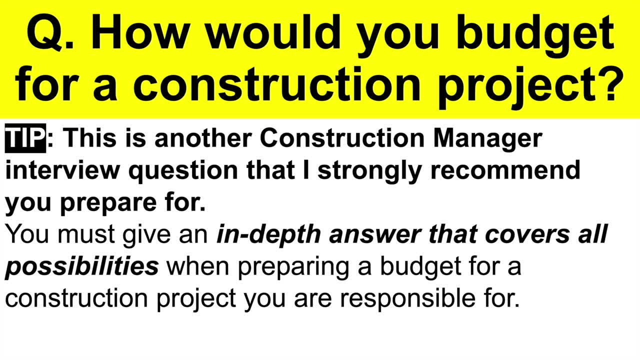 So it's another construction manager interview question that I strongly recommend you prepare for. You must give an in-depth answer that covers all possibilities when preparing a budget for a construction project that you are responsible for. So here's another brilliant template example answer to assist you: How would you budget for a construction project? 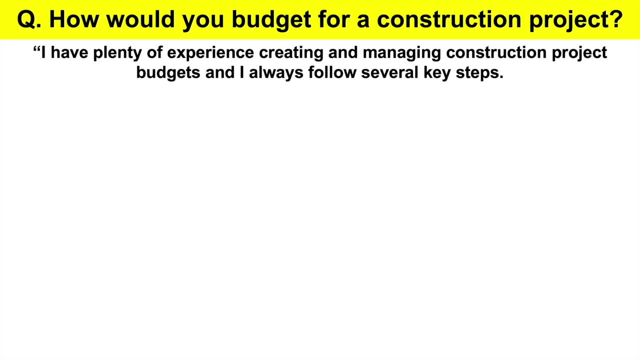 Here we go. I have plenty of experience creating and managing construction project budgets and I always listen carefully. I have saved the world, so I don't miss the chance to say something funny If you don't have. I mean you've said: I'm not sure, sure, Just annoyed. but have you thought out all that information, that your 78 seconds every day sent you a comment avec Dieu? Et maintenant je suis conscient de penser sur cette question, Today's interview is coming up: a cute idea from a senior manager who is based on a senior manager. 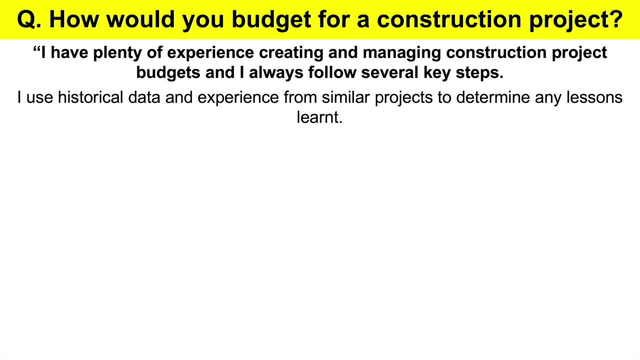 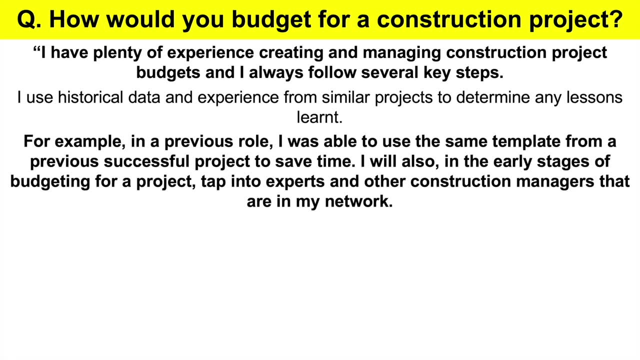 several key steps. I use historical data and experience from similar projects to determine any lessons learned. For example, in a previous role I was able to use the same template from a previous successful project. to save time, I will also in the early stages of. 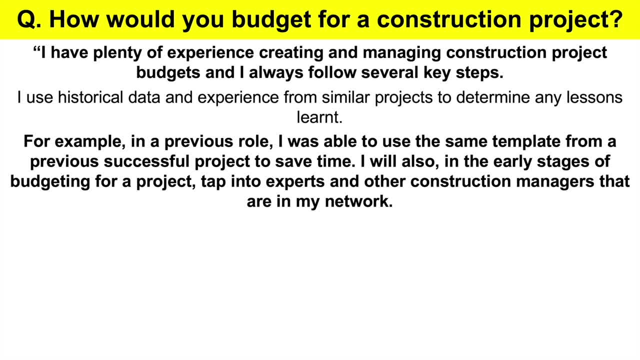 budgeting for a construction project. tap into experts and other construction managers that are in my network. Just a simple phone call to a colleague in a different organization can save me hours worth of research and time. I would then assess the various costs both. 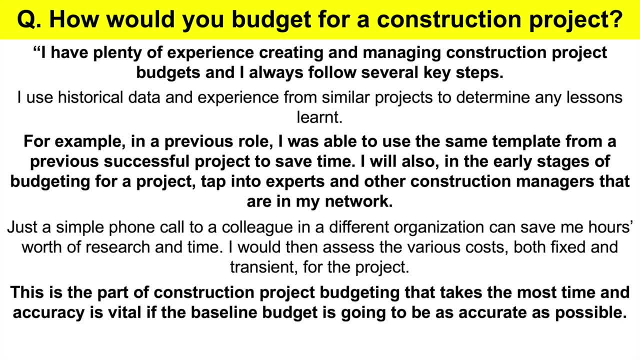 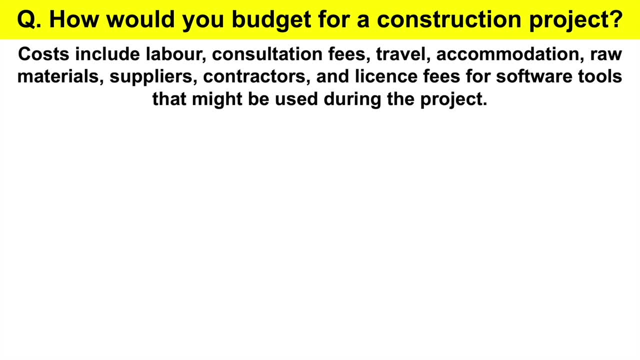 fixed and transient for the project. This is the part of the project budgeting that takes the most time, and accuracy is vital if the baseline budget is going to be as accurate as possible. Costs include labour, consultation fees, travel, accommodation, raw materials. 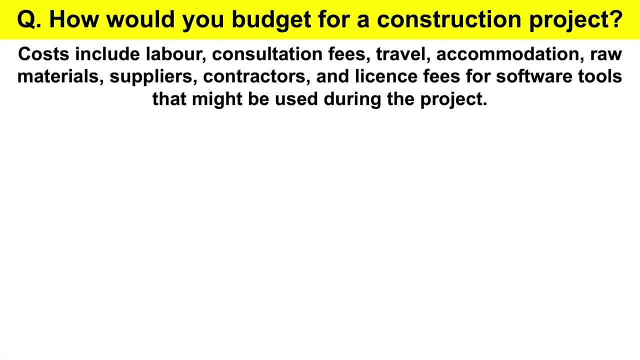 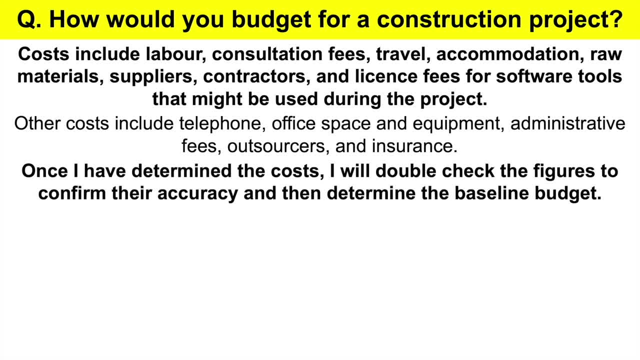 fees, outsourcers and insurance. Now, once I have determined the costs, I will double check the figures to confirm their accuracy and then determine the baseline budget. Now, the baseline budget is likely to change as the project progresses, and it will need to. 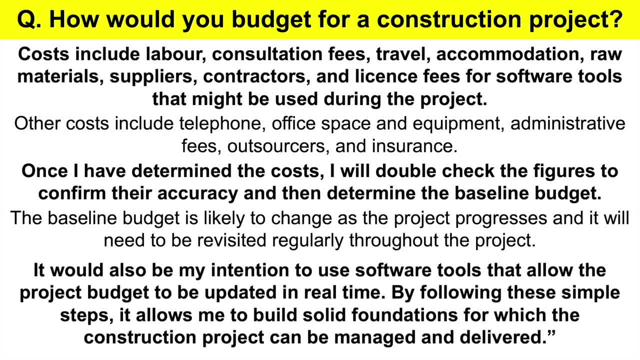 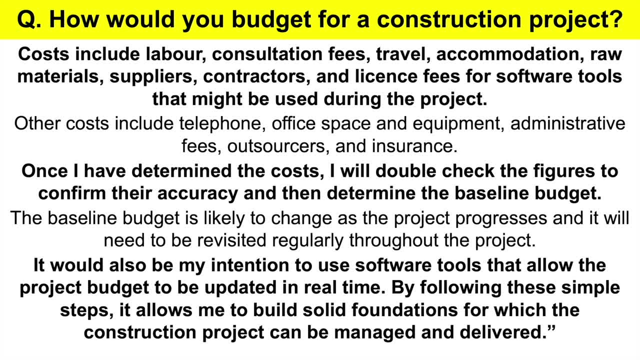 be revisited regularly throughout. It would also be my intention to use software tools that allow the project budget to be updated in real time. By following these simple steps, it allows me to build solid foundations for which the construction project can be managed and delivered. That's another brilliant. 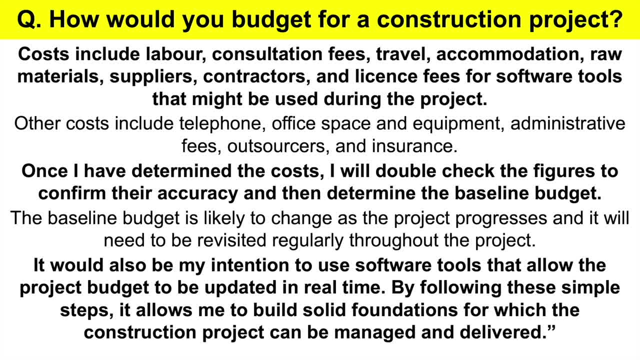 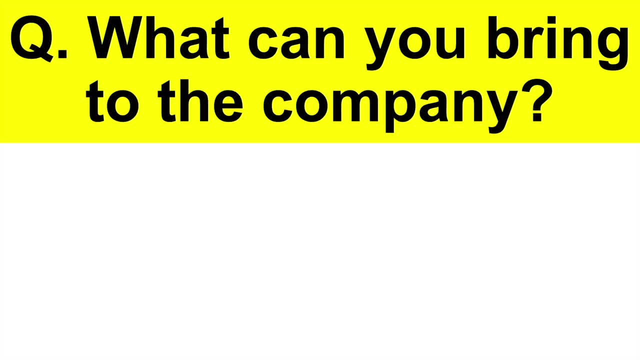 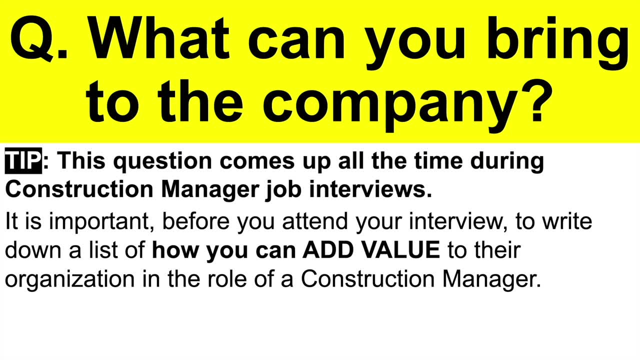 answer that will help you be the standout candidate at your construction manager job interview. Here's the next question that I recommend you prepare for: What can you bring to the company Now? this question comes up all the time during construction manager job interviews. It is important, before you attend your interview, that you write down: 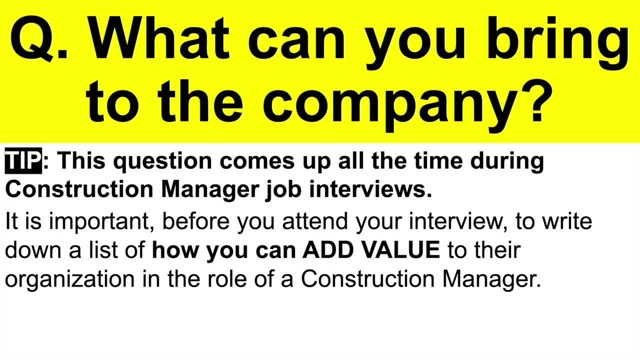 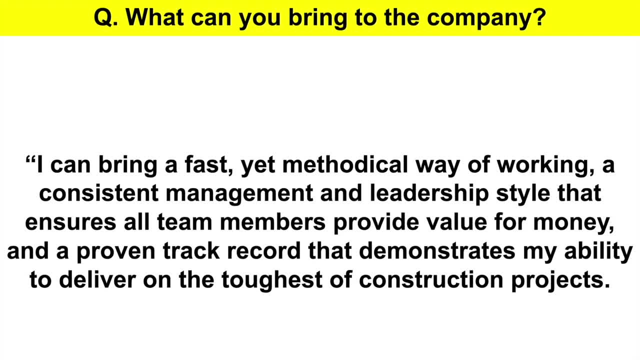 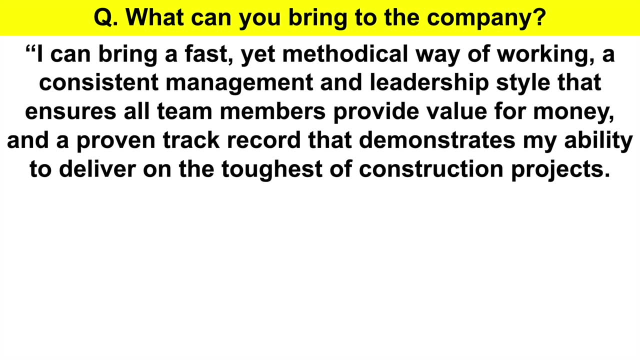 a list of how you can add value to their organization in the position. Here's another brilliant example. answer: What can you bring to the company? Here we go. I can bring a fast yet methodical way of working, a consistent management and leadership style that ensures all team. 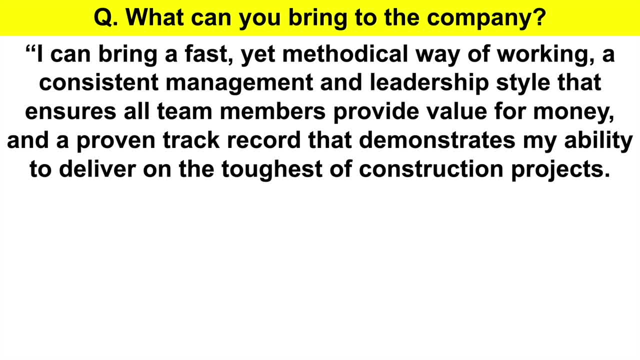 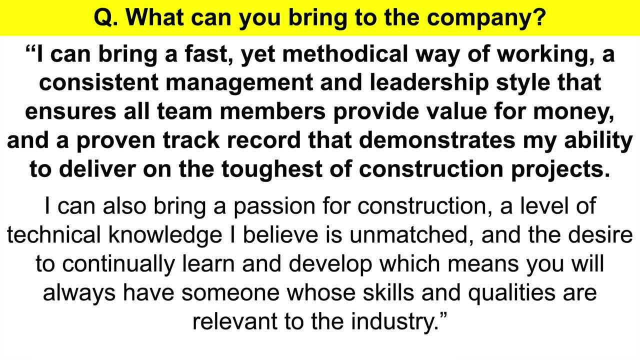 members provide value to the company. I can bring a fast yet methodical way of working, a consistent management and leadership style that ensures all team members provide value for money, and a proven track record that demonstrates my ability to deliver on the toughest of construction projects. I can also bring a passion for construction, a level